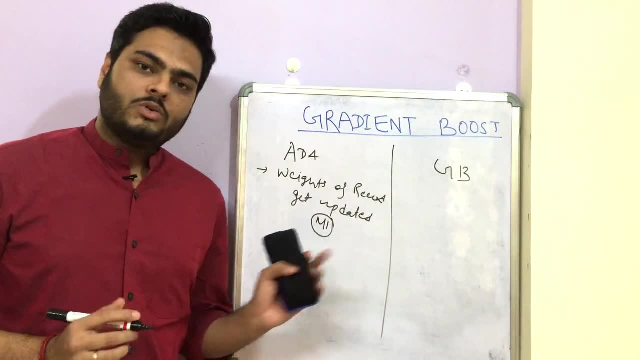 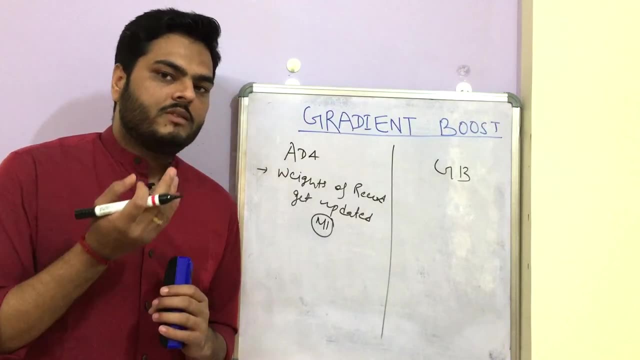 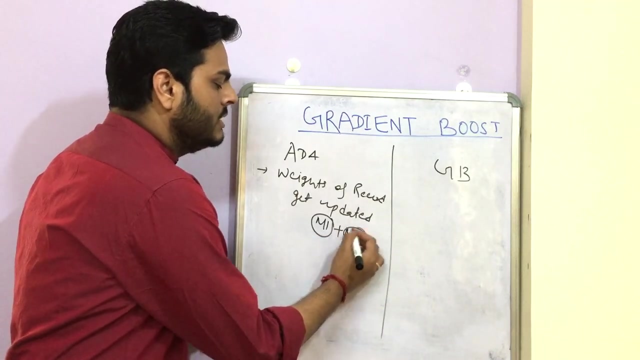 one misclassifies some of the records, or model one is not able to, you know, correctly predict some values or the error is high, then those records will be given more weightage in the next iteration, And this continues. So final model is model one plus model two plus model three. 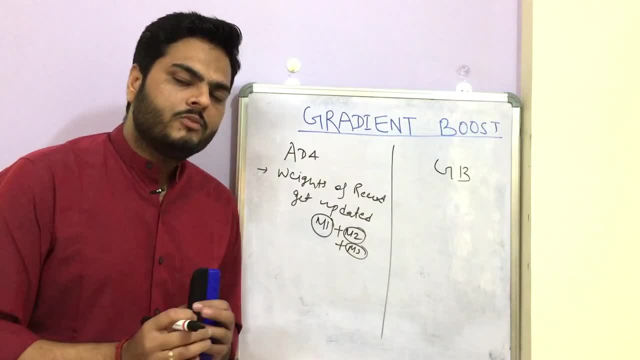 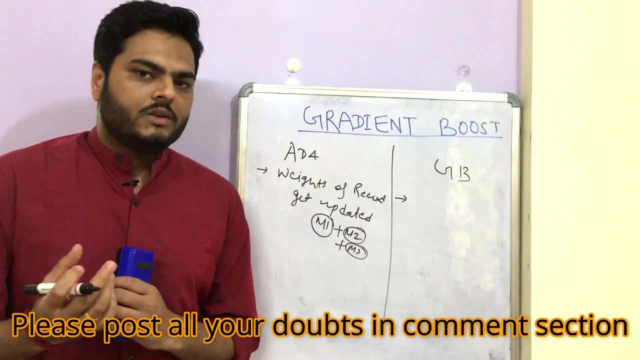 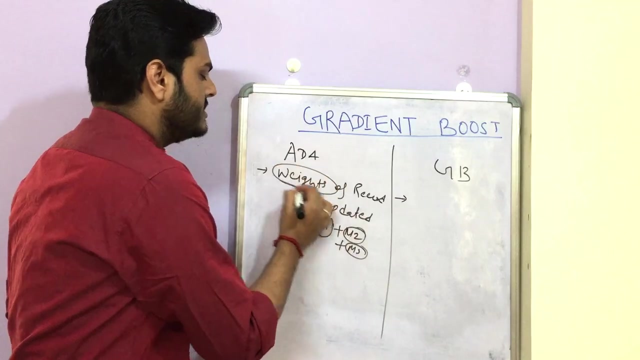 So this is how AdaBoost works. So all boosting algorithm work on combining multiple models. Here also in gradient boost also, multiple models will be combined. So what is the difference? The difference is here: the learning happens by adding the weights, right. So, as I told, 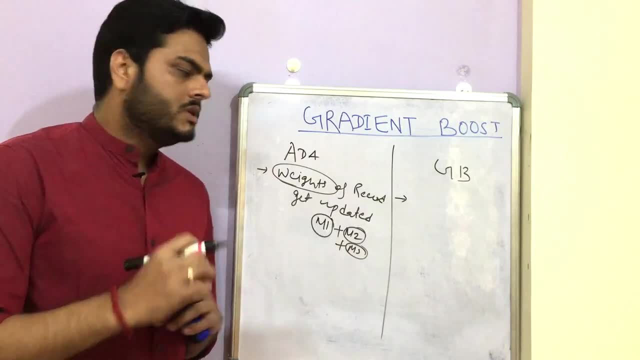 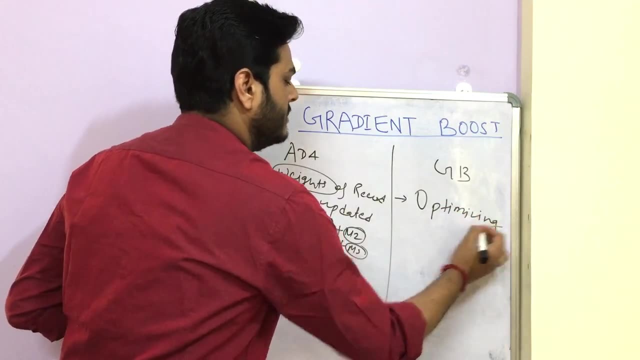 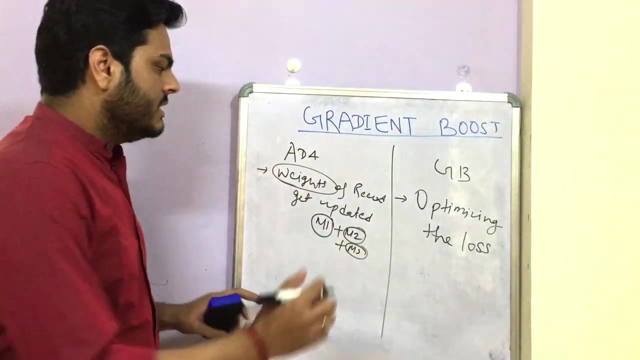 learning happens by changing the weights. In gradient boost, learning happens by optimizing the loss function, optimizing the loss. So what is this loss? I'll talk about this in a moment. Before that, the another difference between AdaBoost and gradient boost is in AdaBoost, the trees- normally the trees which 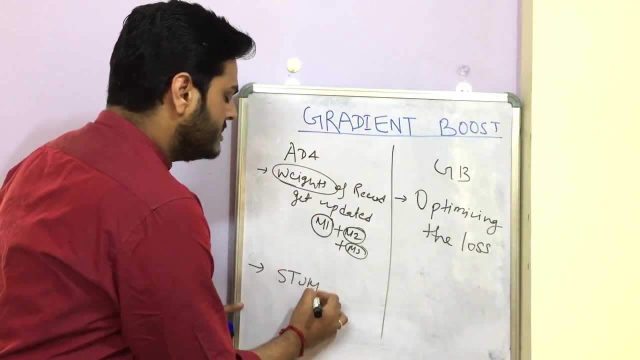 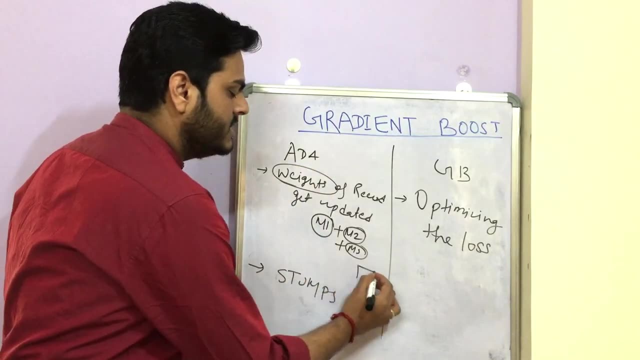 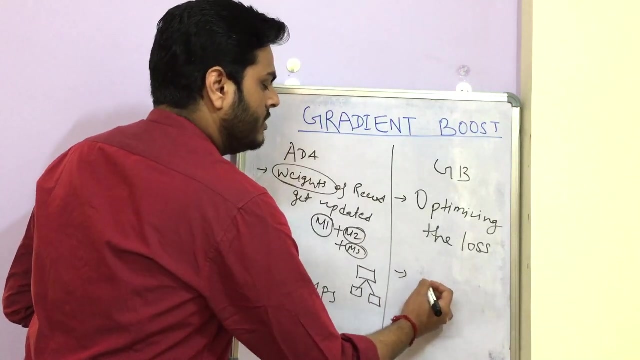 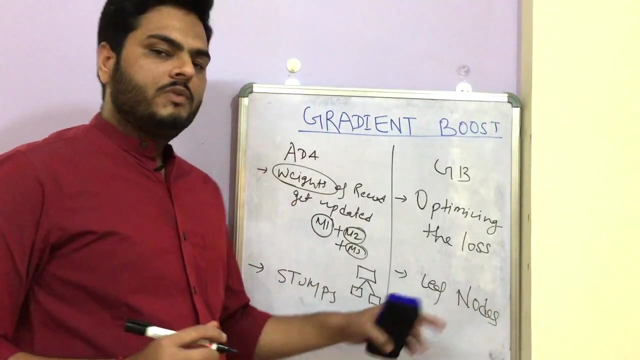 are built are basically stumps, which means trees are not grown fully or trees are not grown below a limit. So trees normally look like this: 1 root and 2 leaves, Whereas in gradient boost the trees are normally leaf nodes. So here there are only two leaf nodes, Whereas in gradient boost the leaf nodes will be. 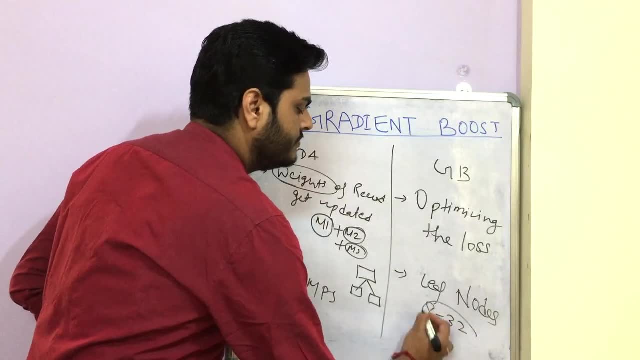 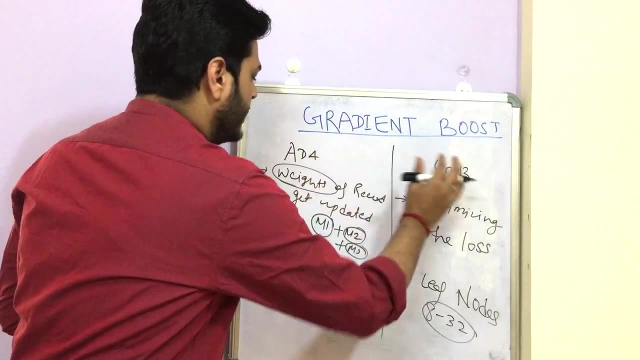 only the range of leaf nodes between 8 to 32, which means that trees are bigger in size in gradient boost. So there are two differences between AdaBoost to gradient boost. And what's this load? It's not everything, So there is no load either. On input, input, input사�ing and output, infertility isn't required. 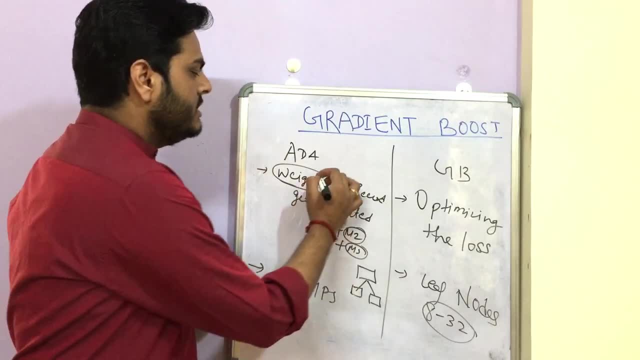 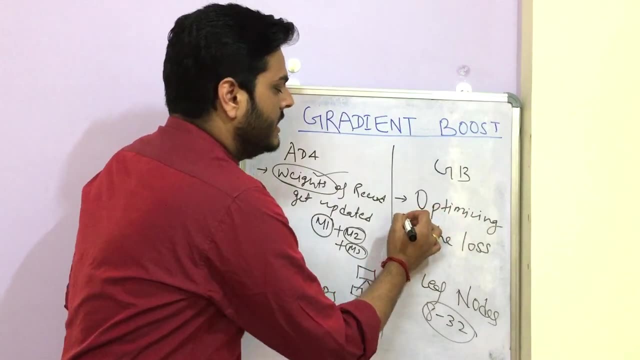 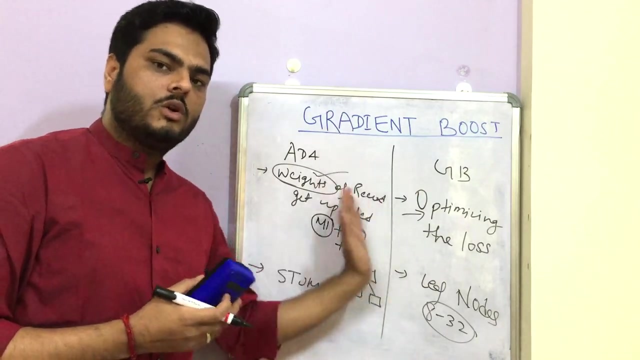 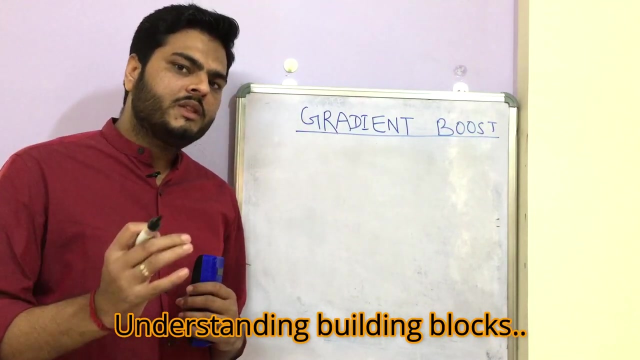 or you know, the boosting happens by adjusting these weights of the records, misclassified records. on the other hand, in gradient boost the learning, or you know, assembling happens by optimizing the loss. now let me talk a bit about what is loss. if you guys remember how linear regression works using ols method, ordinary least square method, then you will be able to recollect. 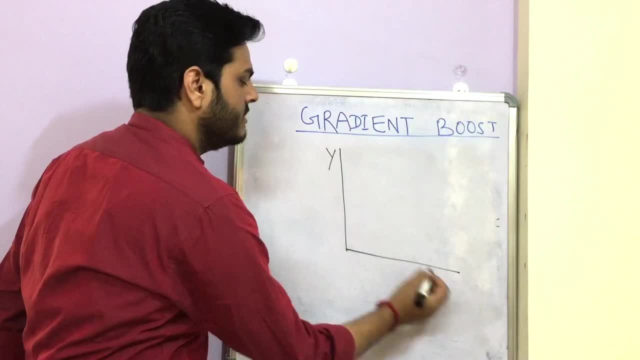 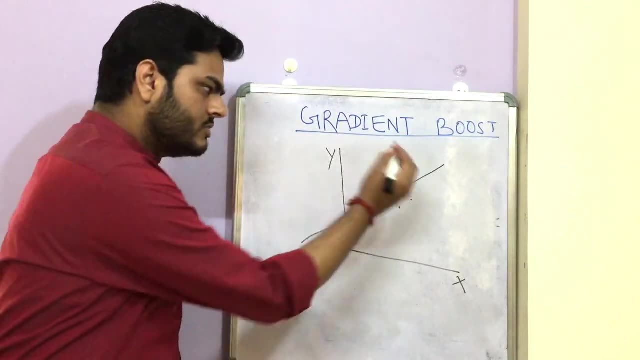 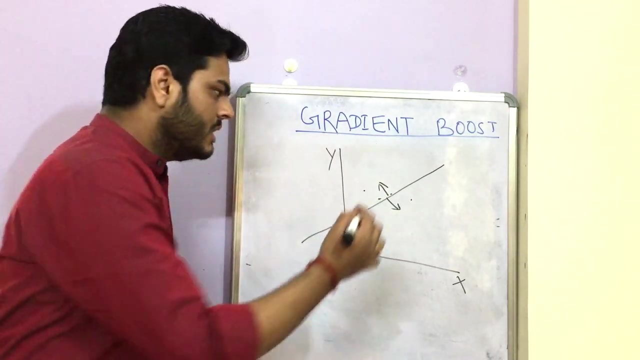 that in linear regression, if this is y axis and this is my x axis, if these are my data points and this is my regression line, then the errors of this regression model are these distances- distance between actual values and predicted values- right, and we call these errors as e1, e2. 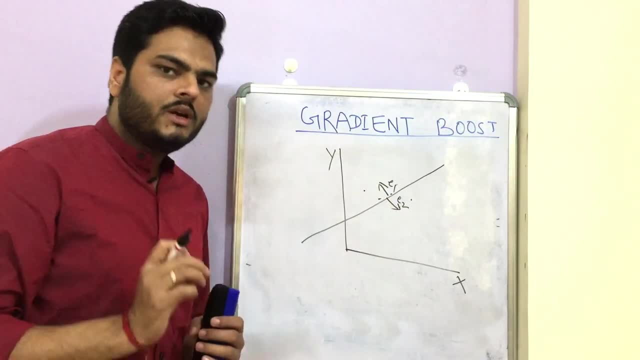 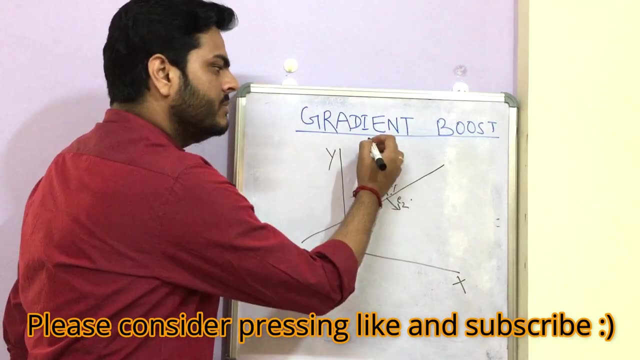 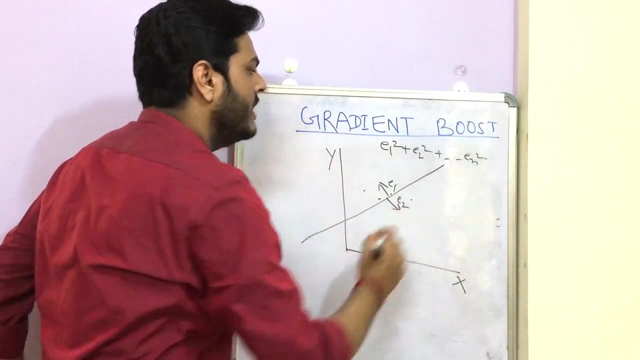 like this. so how ordinary least square method, or ols method, works is by optimizing these errors. so what is the meaning of that? the, the, the ordinary least square method, tries to optimize e1 square plus e2 square plus up to en square. why we are squaring this is because some of these can be negative and some of these can be positive. 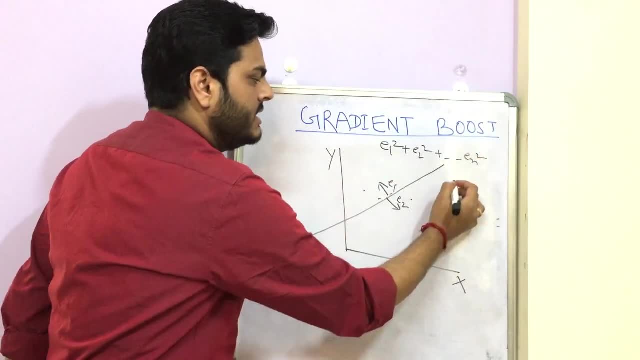 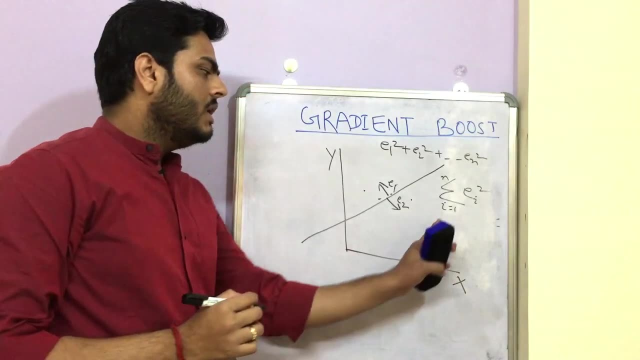 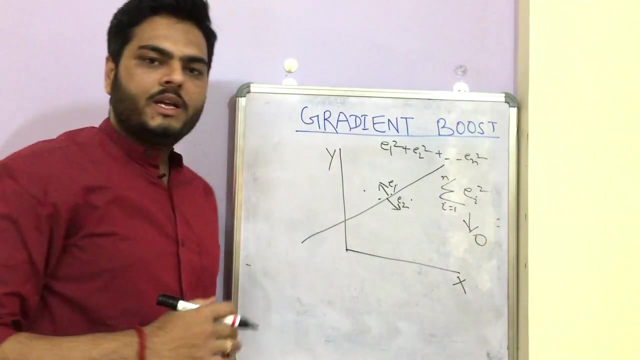 so we can make this equation generic with a summation. we can say: i is equal to 1 to n and ei square. so how ols will work? is ordinary least square in linear regression. it will try to bring this value as close to 0 as possible. 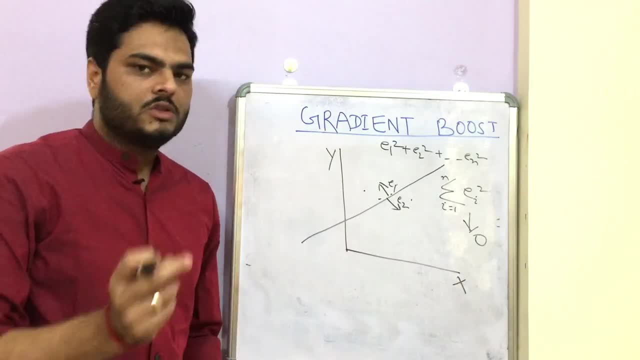 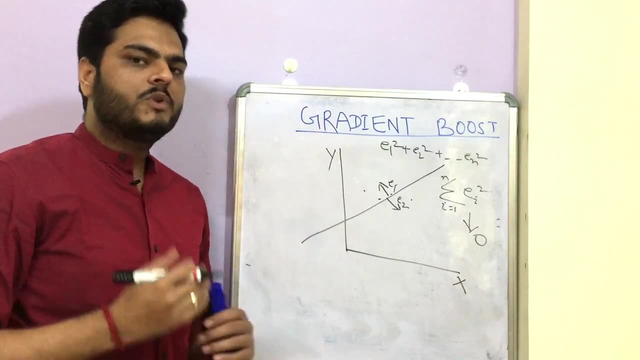 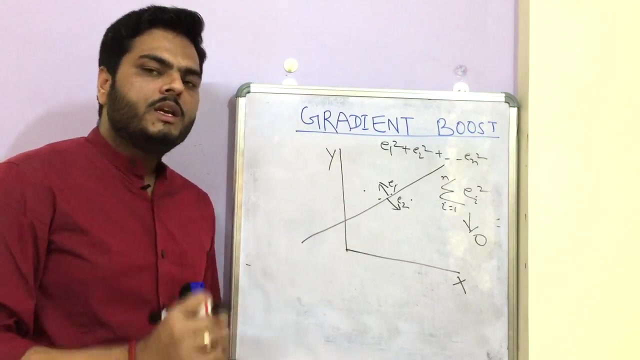 and this process is called optimization of loss function. now, what is loss function? this becomes the loss function for this particular model. okay, and this process is called optimization of loss. now, why this is important is the same concept is being used in gradient boost as well. let's try. 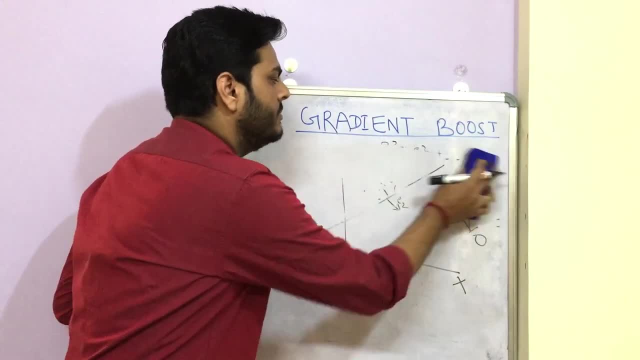 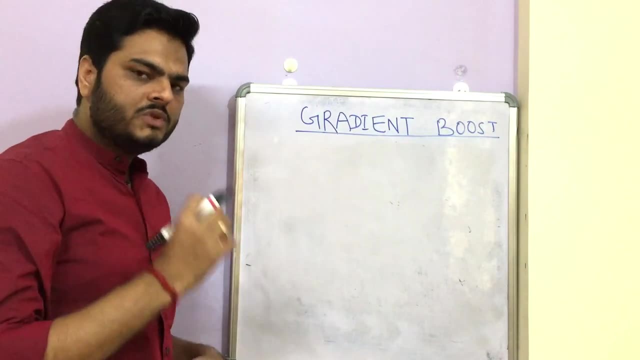 understanding. how is that? okay, so i will take a very simple data here and try to make you understand how gradient boost works. okay, just pay attention, guys. gradient boost is very simple. so gradient boost works here. only its a shape of a shape, a shape of a circle. you se perfectly. but if we consider gradient boost, 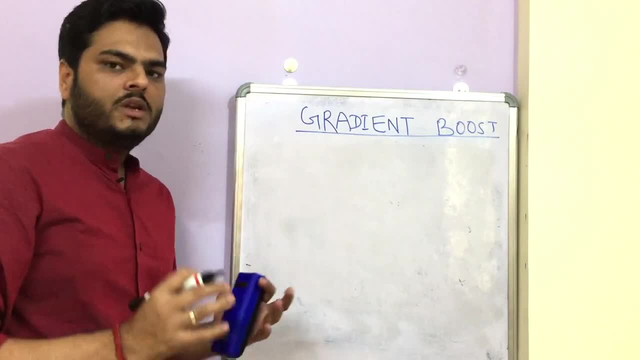 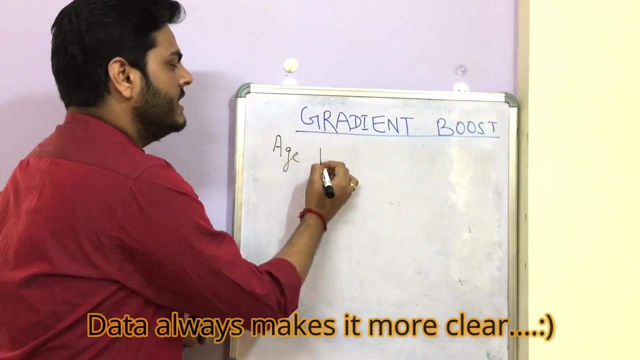 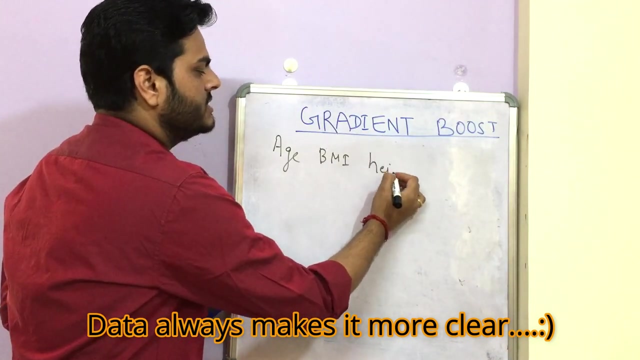 is something which is not very well explained on internet and web. okay, so just pay attention here. so let's say, i take the age of a person, i take the bmi of a person and let us say, from age and bmi i want to calculate the height of the person, or i want to learn this pattern. okay, now let me put. 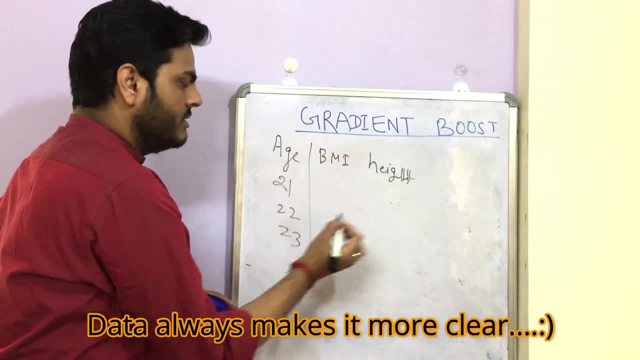 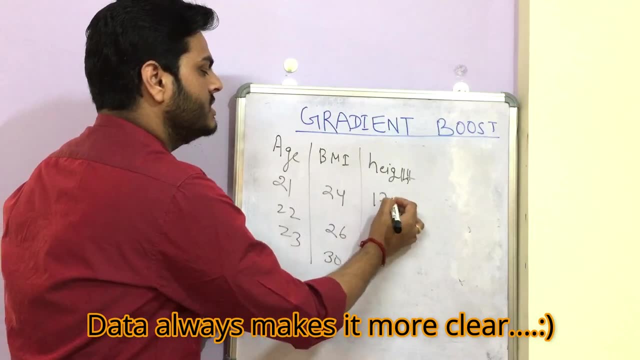 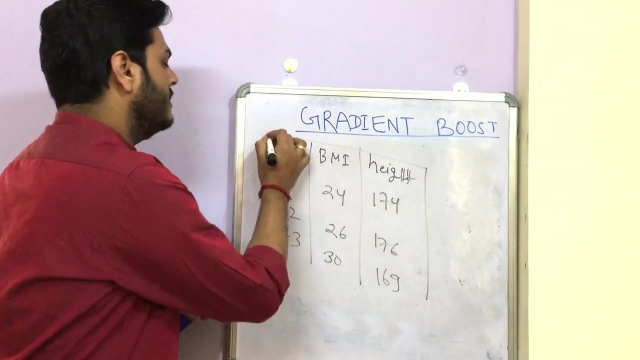 some rambas here: 21, 22, 23, bmi might be 24, might be 26, might be 30 and let us say, height might be 174, 176, 169, something like this. okay, so let us say in this data, these two age and bmi are my. 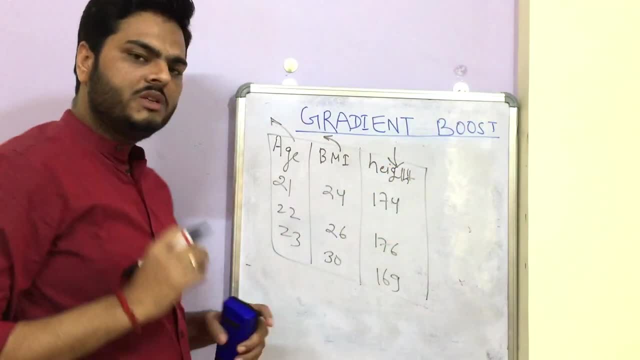 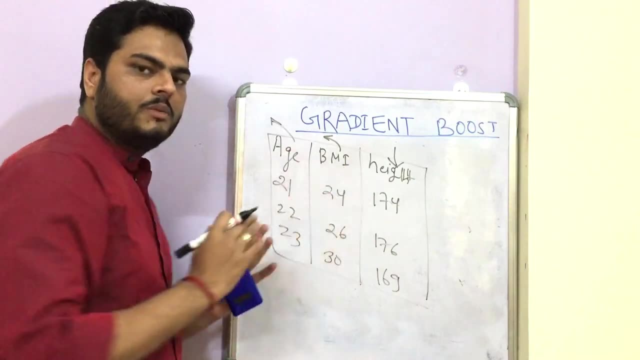 independent variables and this is my target variable, which means this is a regression problem. so we want to learn the pattern- how height is different from age and bmi- and we want to learn the pattern how height is different from age and bmi. okay, so this is what we are interested in learning now, if we take this data and submit. 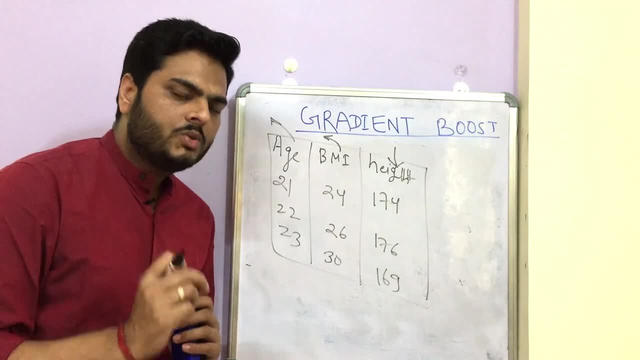 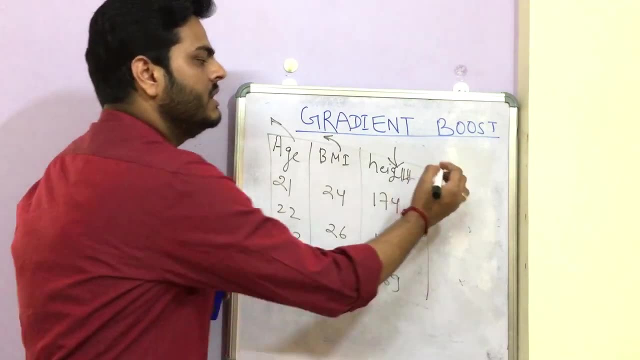 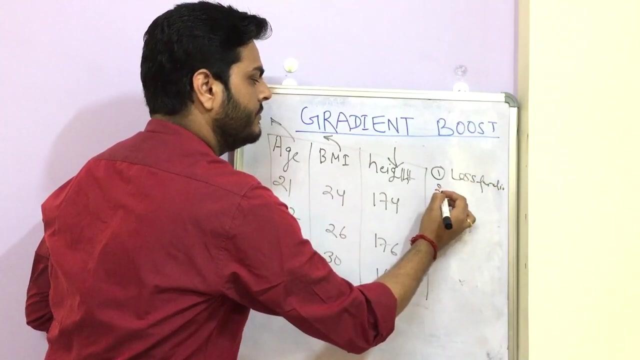 this data to a boosting algorithm. so let me walk you through, step by step, how boosting algorithm will work. so the very fundamental thing in boosting algorithm is it will need two things. one is a loss function- okay, and another is a additive model- okay. so i'll tell. 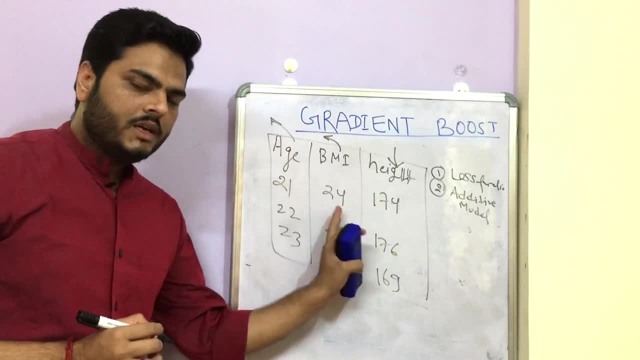 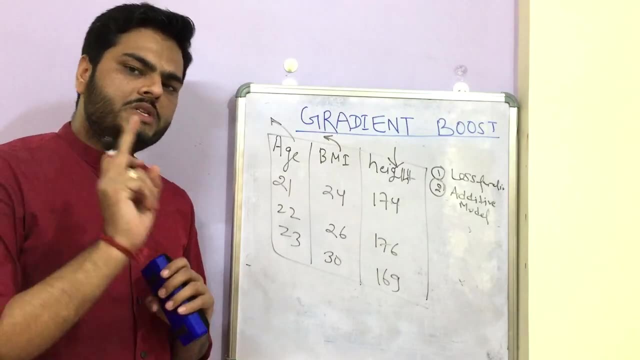 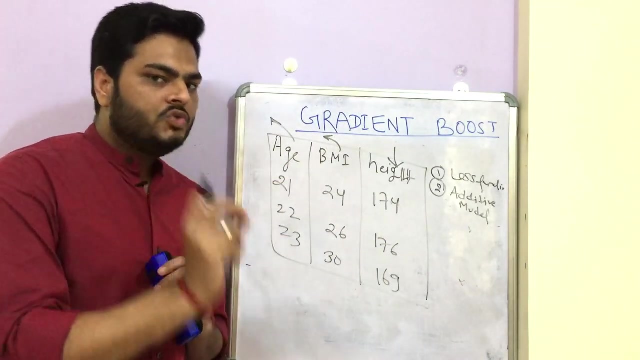 you what are these things in a moment now, this is the data. so the very first thing the boosting algorithm does is it will try to compute the first residual. so what is residual? if you remember, in linear regression i just discussed, residual is the difference between actual value and predicted. 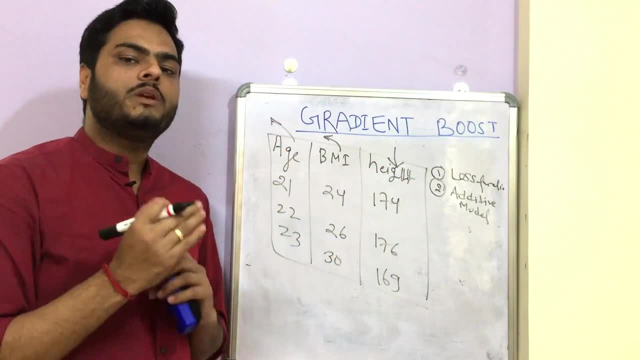 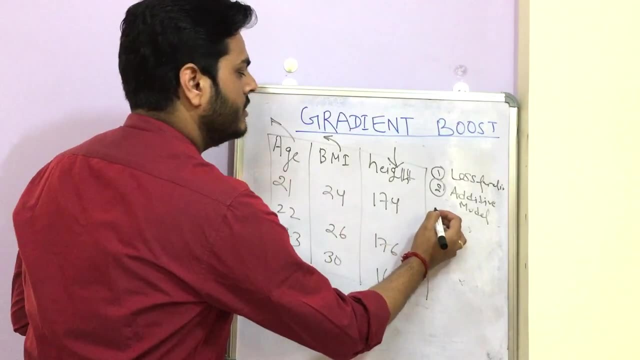 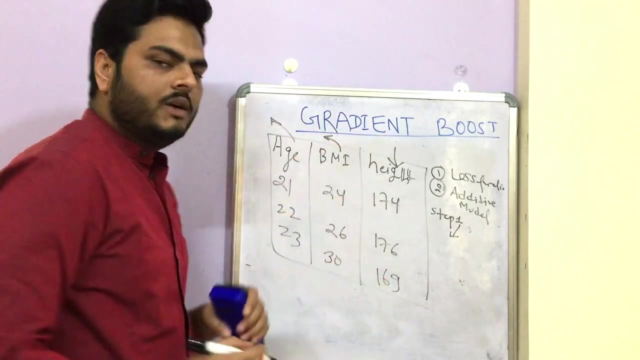 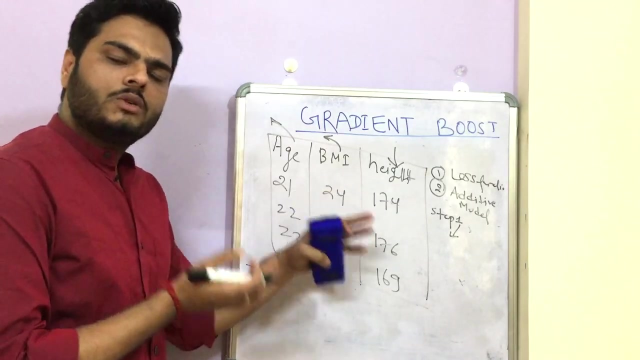 value. in this context, we do not have any predicted value. so where from the residuals will come? so what boosting algorithm does is in step one, or you can call it step zero. in step one, boosting algorithm will just compute the average of the target column. this happens if it's a regression use case. if it's a classification use case, then the concept 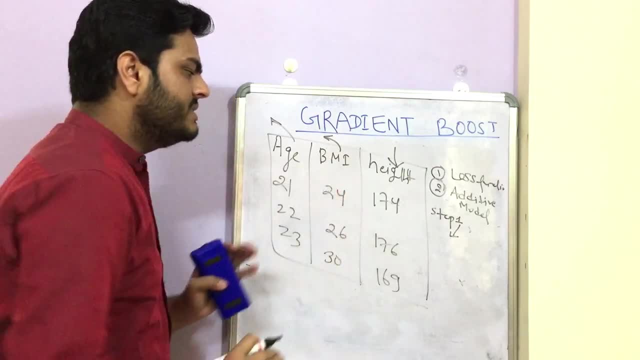 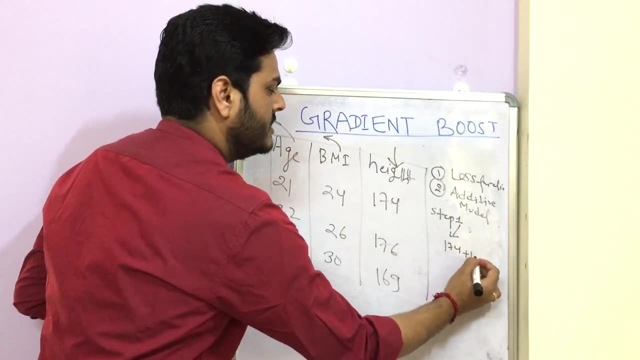 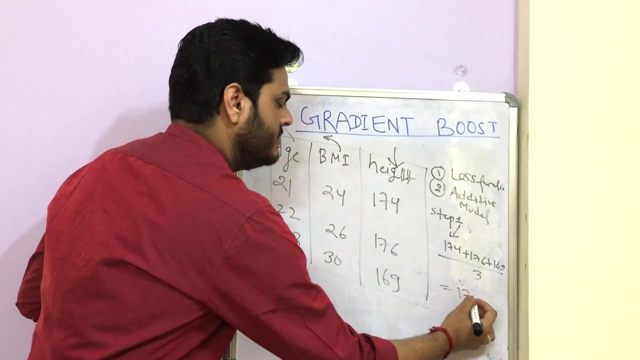 of odds and probabilities will come. okay. but here, to keep it simple, let's try understanding what is the average height of this, so we can say: 174 plus 176 plus 169 by 3. okay, is equal to, let's say- i'm just putting a dummy number here- if it is 171, i'm not sure if this is the right answer. let's go with that, okay. 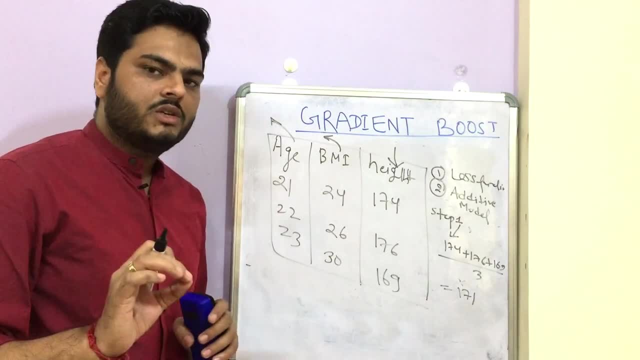 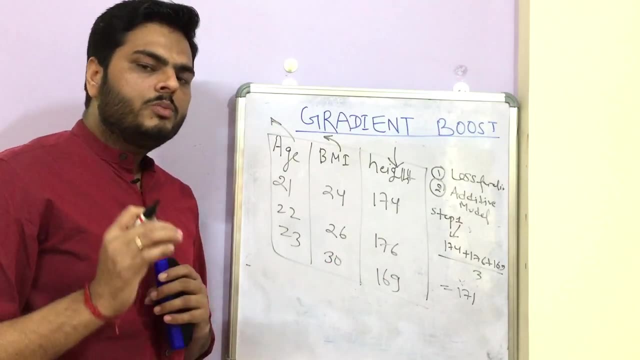 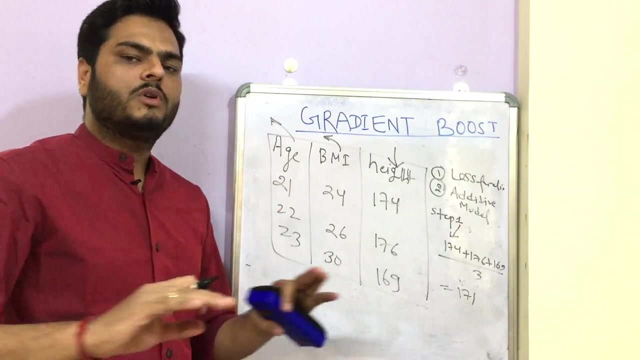 so 171 is the average height of this column. now what happens if there is no model, no learning in place? so boosting algorithm in step one assumes that there is no learning in place or no model, which starts with the base model, no model at all. then what will be the predicted values of this? 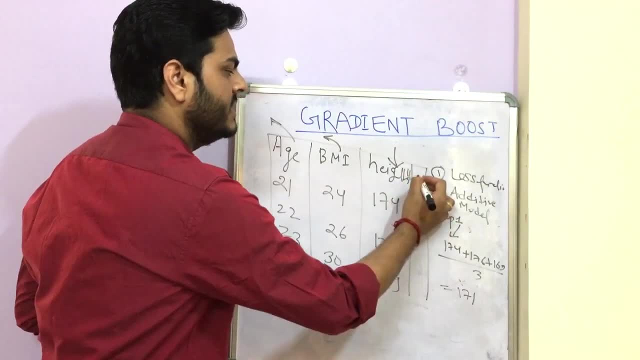 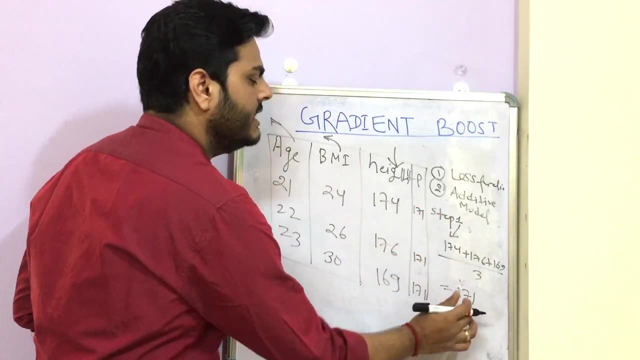 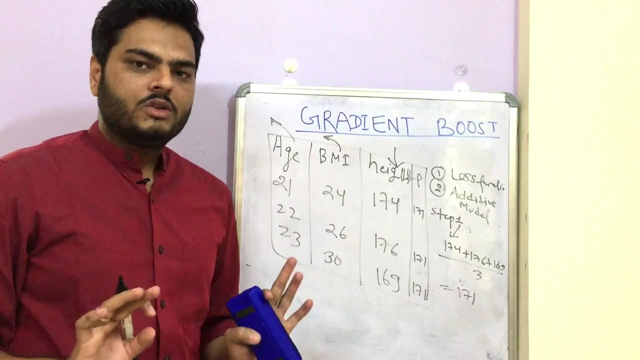 so if i have to add predicted values here, then all the predicted values will be 171, whatever we have computed the average here. okay, this is step number one. this is step number two. now we have actuals and we have predicted, so we can have the residuals. okay, so what will be residuals here? actual minus predicted. so this: 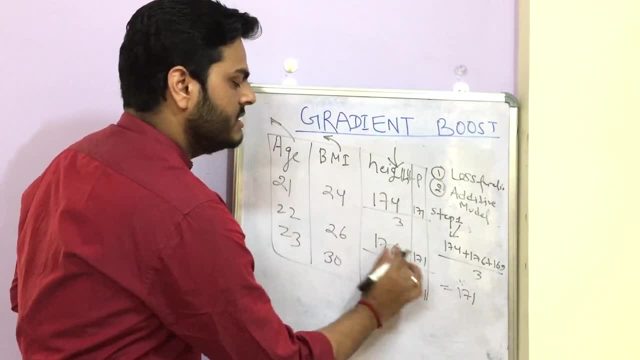 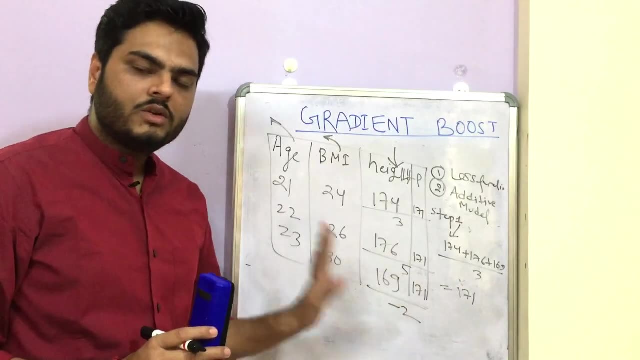 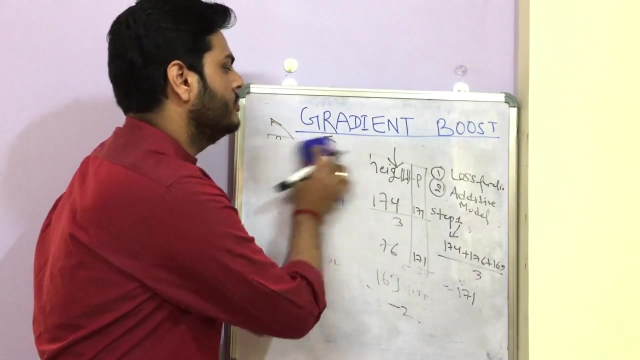 residual will be three. what will be residual? well, this residual will be five and this residual will be minus two. okay, now we have residuals in hand. okay, this is step number one. step number two: now i am rubbing this off, just. you can go back and see the data if you want. 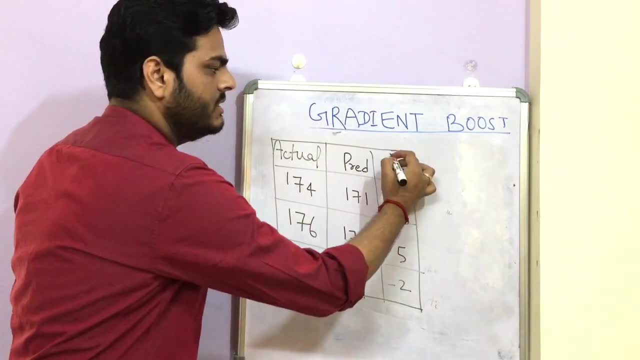 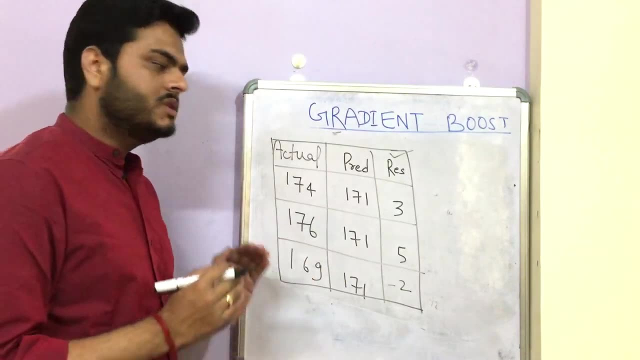 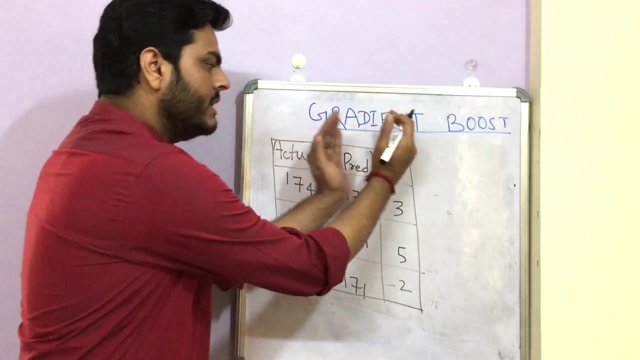 so these are the actuals, these are the predicted and these are the residuals. okay, having said that, as a next step, what gradient boost will do is gradient booster will fit a model on this particular residual. so residual becomes the target column and all the individual columns of this particular column will consider these residuals in hand. so let's see, this is step number one. step number two: 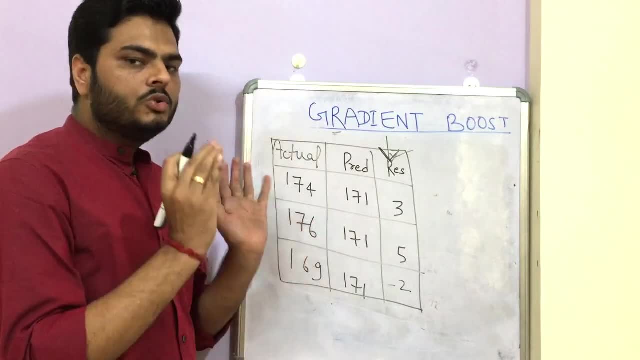 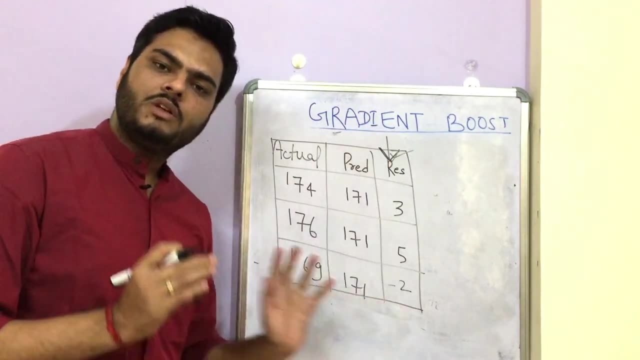 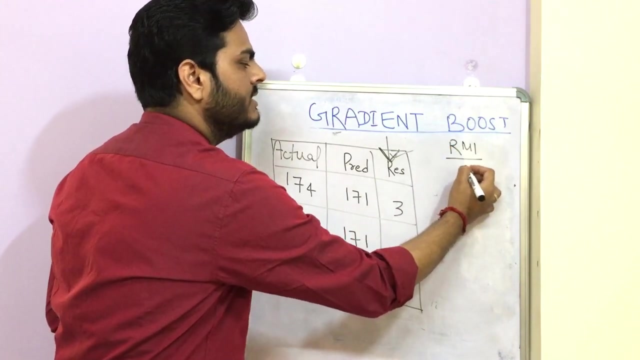 of the data which I have rubbed off: age and BMI. those will be there as independent column and this residual becomes the target column and a model is fit on this residual, So let's call it residual model 1.. Now how this residual model will look like is, let us say, this is decision tree. 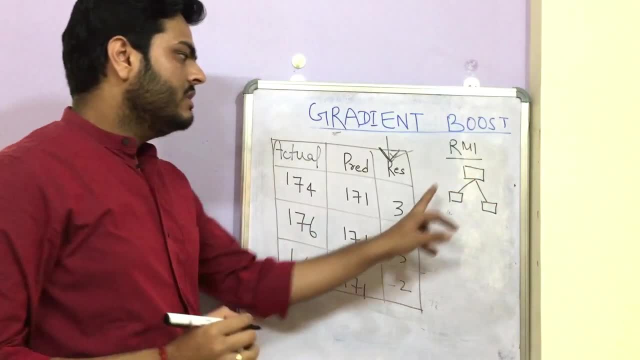 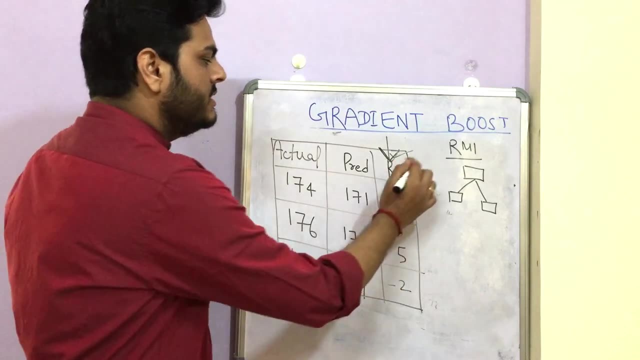 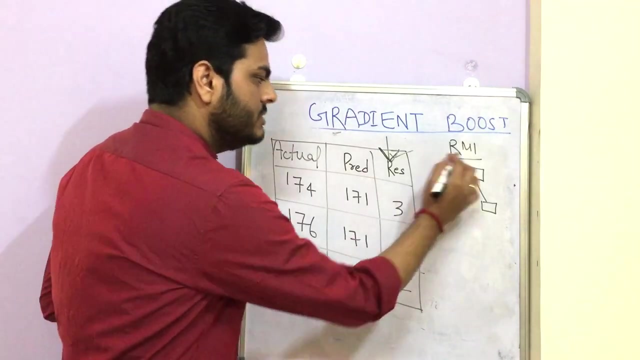 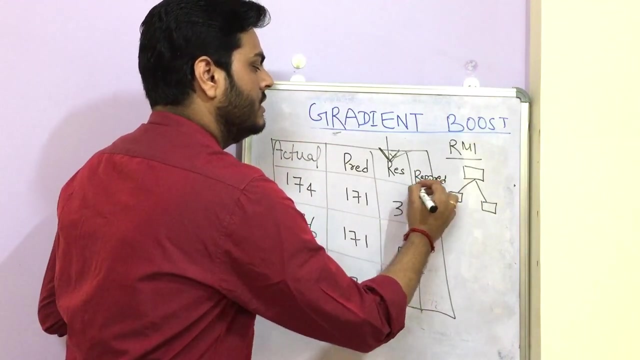 it looks like this, and this residual model 1 is fit on this as residual as target. As a next step, what will happen is these residuals will be predicted using this model. Now, using this model, we will get the new value of the residuals residual predicted. So let us say this model. 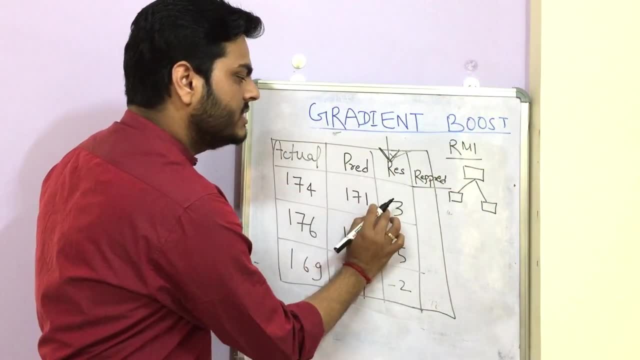 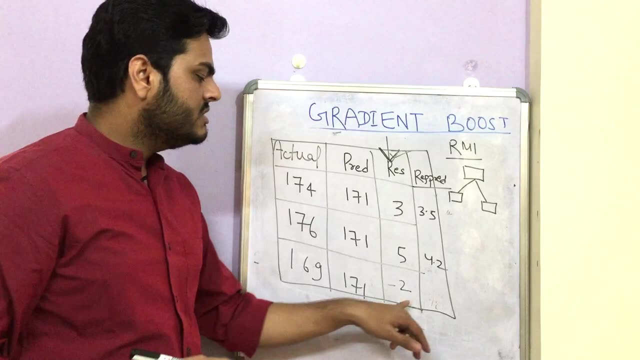 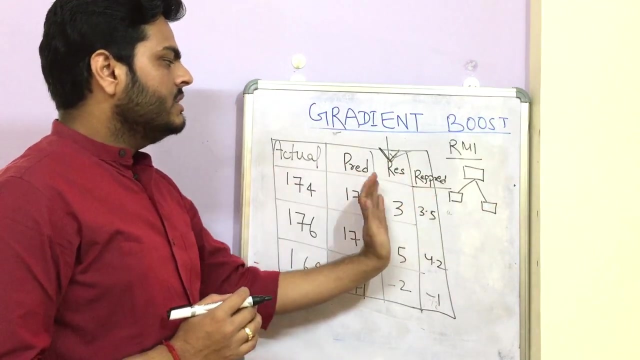 learning happens. and then the value predicted for this residual 3 is- let us say 3.5. for this residual 5 is, let us say 4.2. for this minus 2 is minus 1.. I am just putting some dummy numbers here. So this model is predicting the value of residuals. this 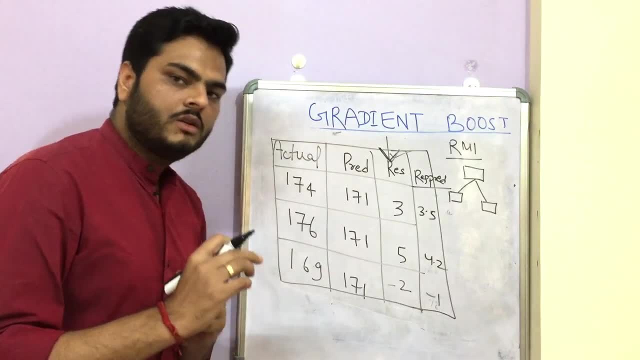 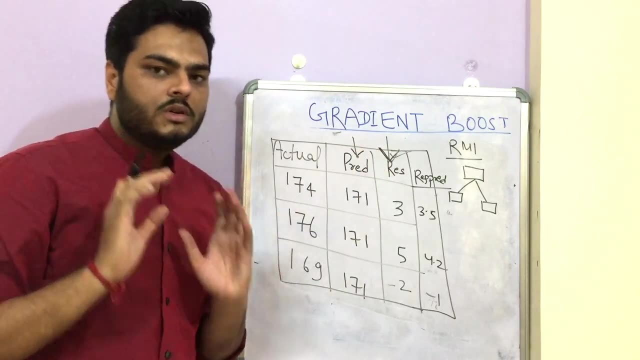 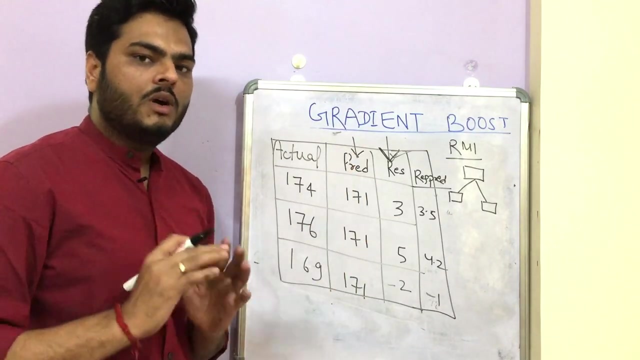 Now what happens, as next step is the prediction gets changed, which means, if you remember, this column is just the average of target column in the beginning, step 0.. Here what will happen is this: 171 will change. now How it will change is the new prediction, The new prediction after. 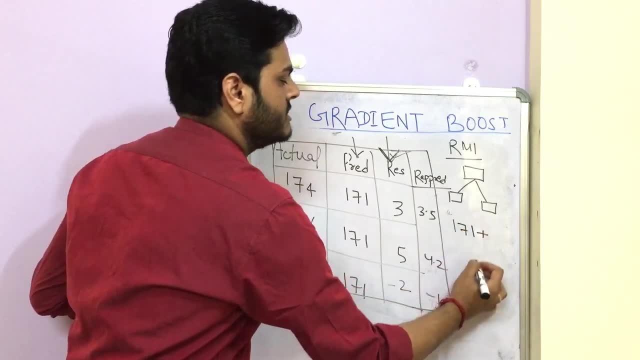 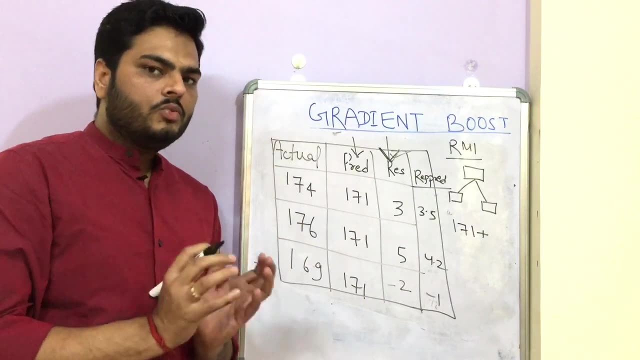 first iteration will change. So the new prediction after first iteration will change. So the new prediction will be 171 plus. there is something called learning rate. So learning rate is the rate at what speed or at what you know shift. you want to change the predicted value. So this value I am. 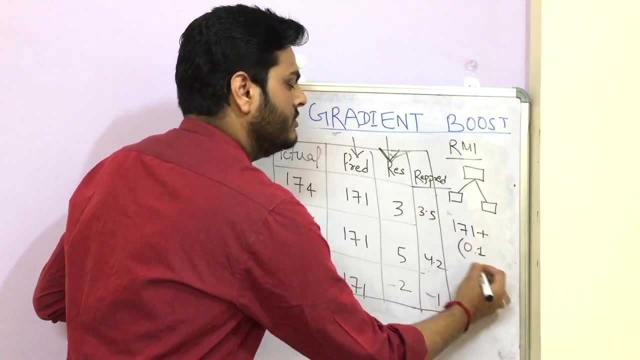 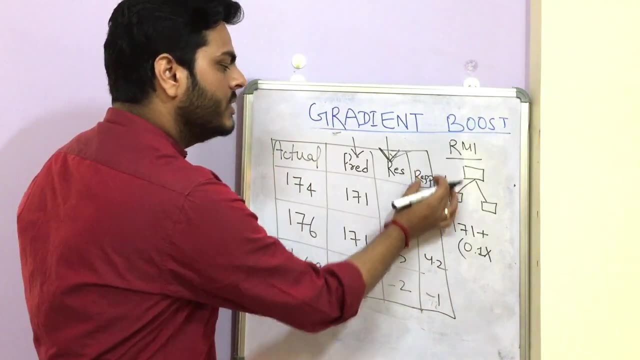 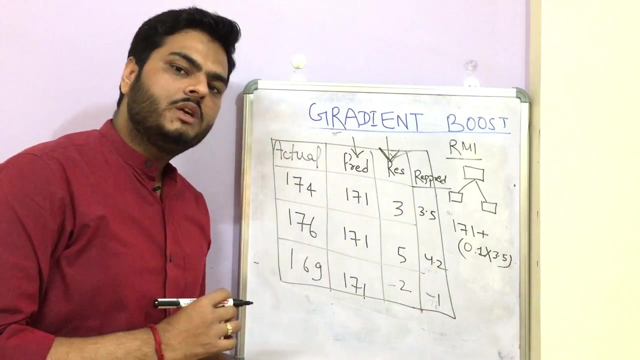 keeping it 0.1 for simplicity. So it will be 0.1 into the residuals difference. So here what is the new residual computed? So this is 3.5.. Now, whatever this output is, this becomes the new predicted value. Okay, If you have some. 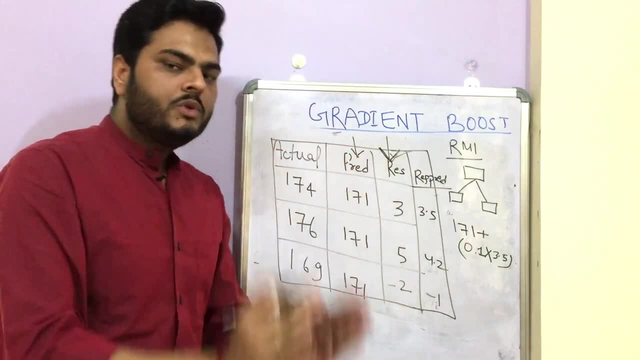 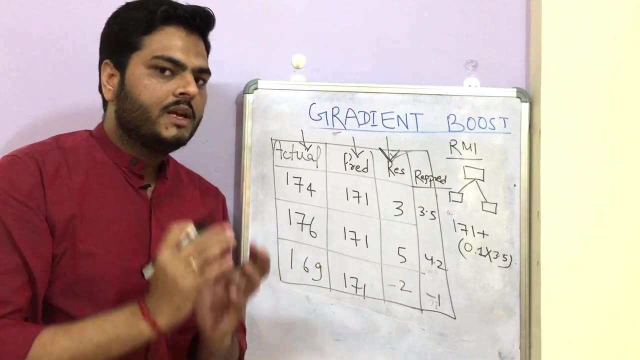 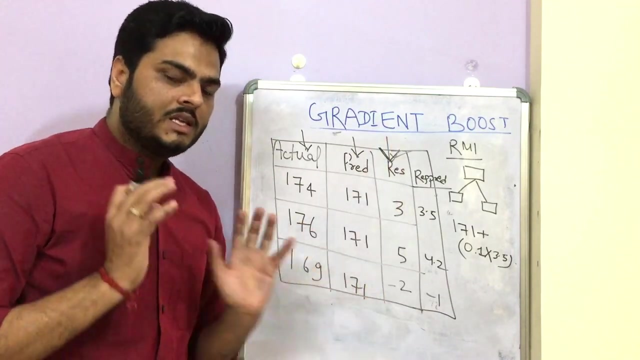 confusions. let me repeat again. Step 1: compute the average of the target column. Step 2: if we have the actual and if we have the predicted, we call that average as prediction. Okay, So actual, predicted, we will have a residual Fit, a model on this, residual as target and independent columns as 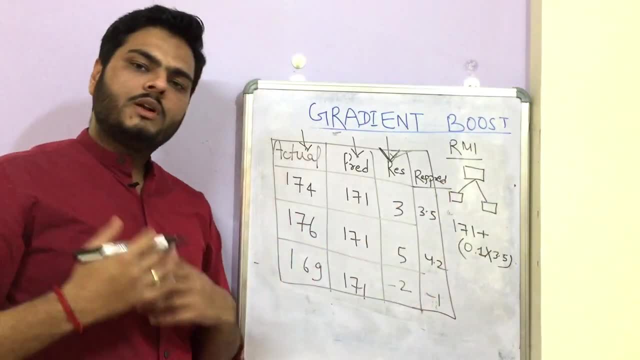 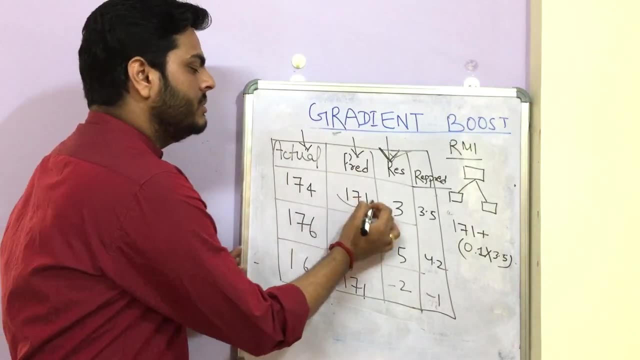 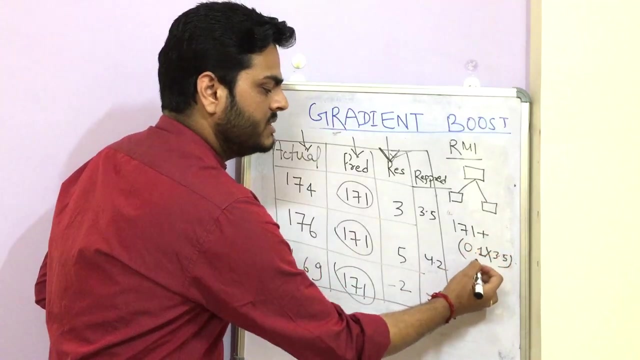 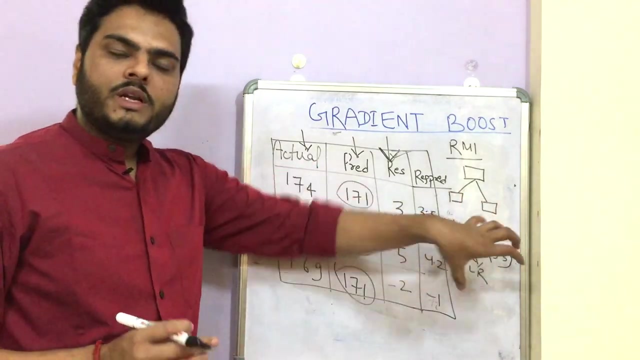 columns of the data Fit a model. This model predicts the residual. Now we have the predicted residual. Now what to do Now? update the default prediction. Okay, So this default prediction 171 gets updated by the new residual 171 plus learning rate into 3.5.. Okay, So this is how iteration 1 gets completed. 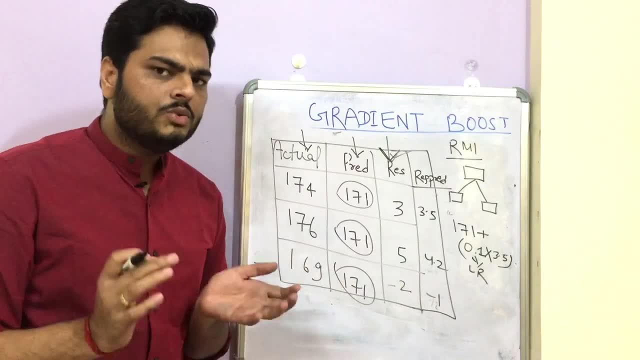 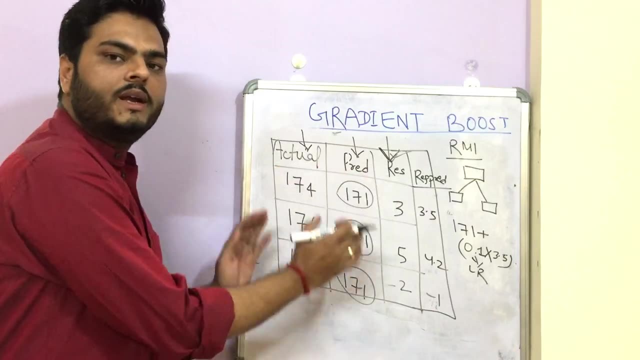 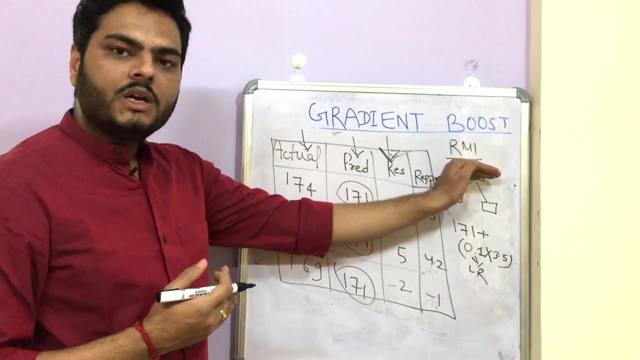 Now we will have new numbers here. Once we have the new numbers, then obviously the residuals will change, because we have the actual value and we have the predicted value, And then residuals will change and the same process will repeat. Okay Again, RM2 will come. Residual model 2 will come. 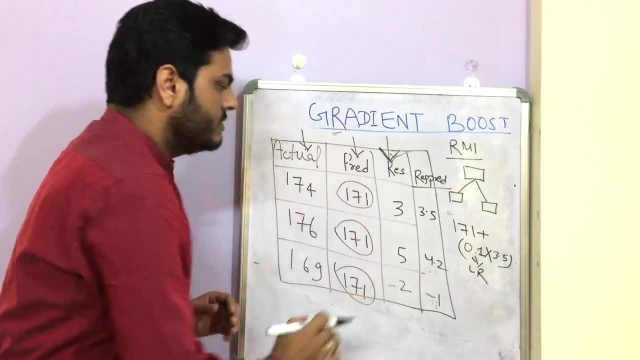 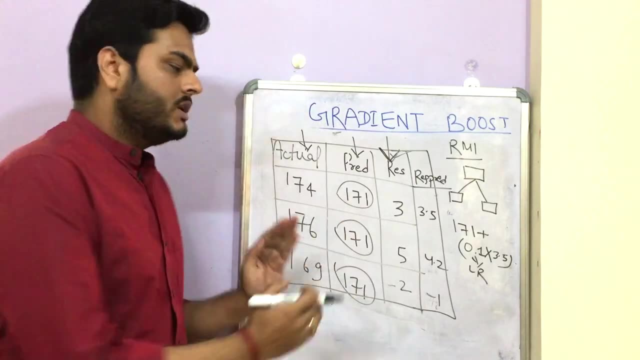 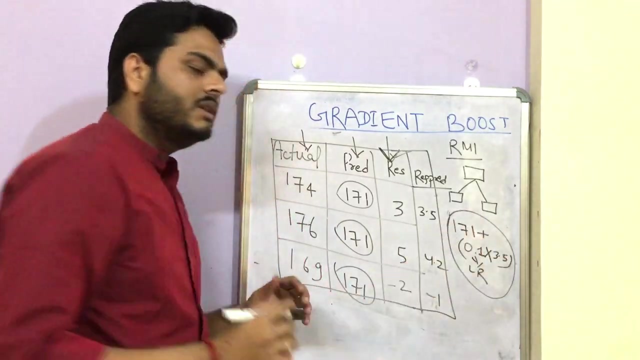 and residual model 2 will update the prediction again. So, if you see carefully, what is being trying to happen here is we are trying to come closer to the actual values. So we made some assumption that this is just the average, Then updating that assumption with the 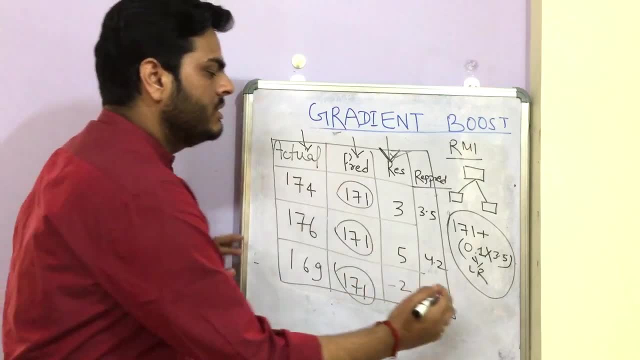 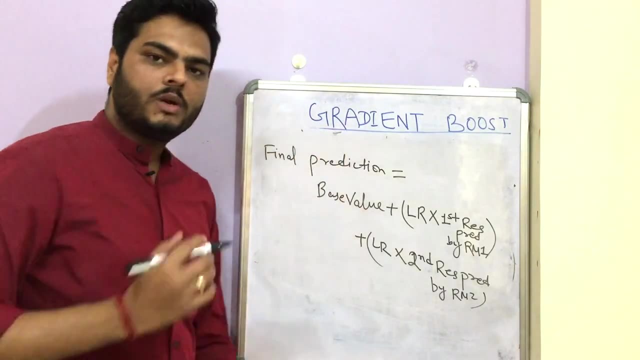 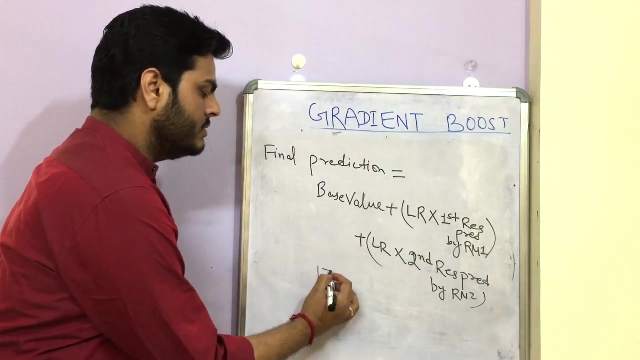 new residual values, then further updating that assumption with one more residual values. so let me show you how the final model will look like. so this is how the final prediction will look like. final prediction will be base value, which in our case is the average value. so let's say that value. 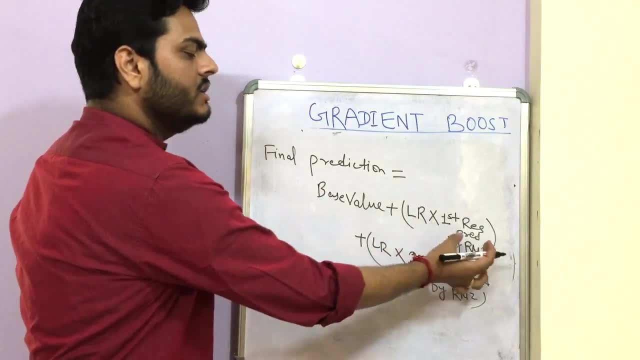 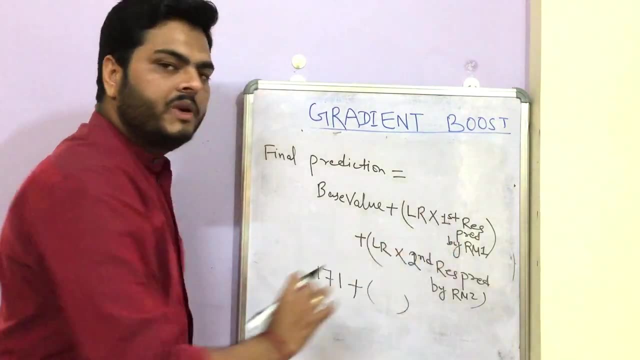 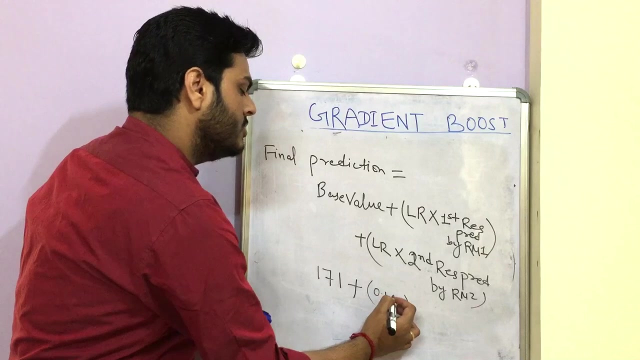 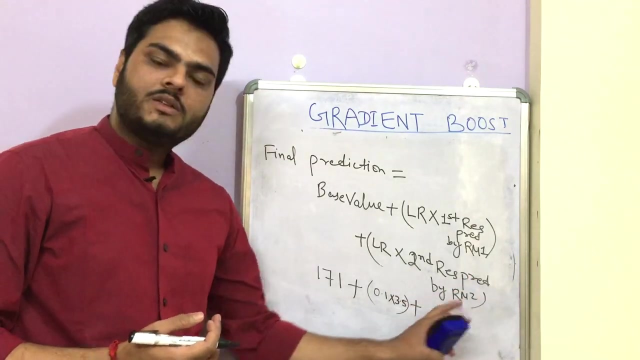 is 171 plus learning rate. into first residual prediction by residual model 1. okay so, first residual prediction by residual model 1. in our record 1 was 3.5 and this learning rate is 0.1. so 0.1 into 3.5 plus learning rate. into second residual prediction by residual model 2.